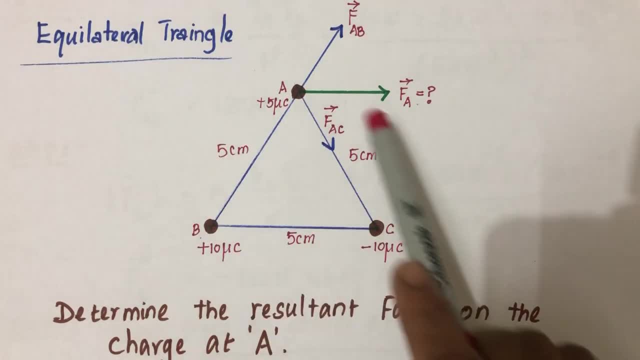 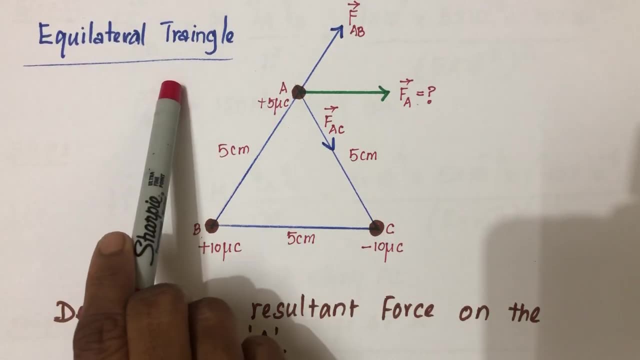 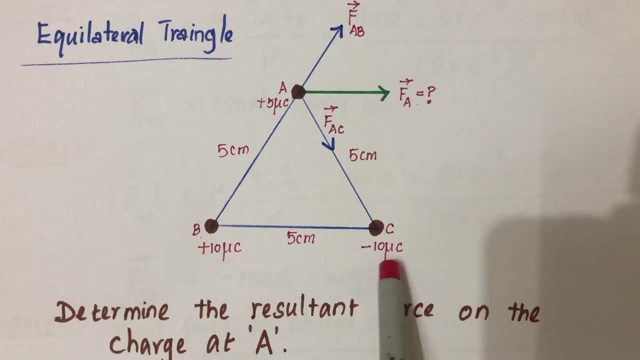 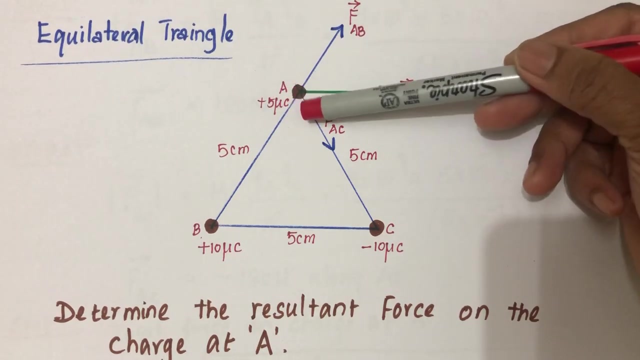 Dear students, in this system of charges there are three charges kept at the corners or the vertices of an equilateral triangle. They are plus 10 microcoulomb. Micro is 10 power minus 6 coulombs, Here negative 10 microcoulomb and here we have 5 microcoulomb at A. 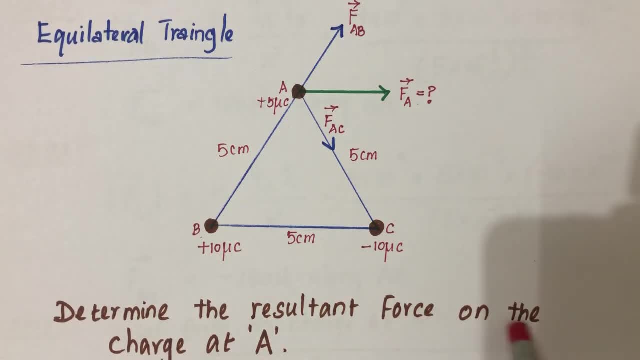 Now the question is: determine the resultant force on the charge at A. So we are going to draw the force vectors at this charge now. So first the charge on A due to B, here plus 10 microcoulomb, and this is also plus 5 microcoulomb. So since both are positive, 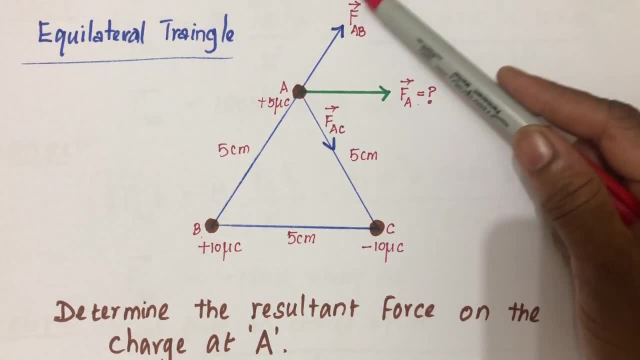 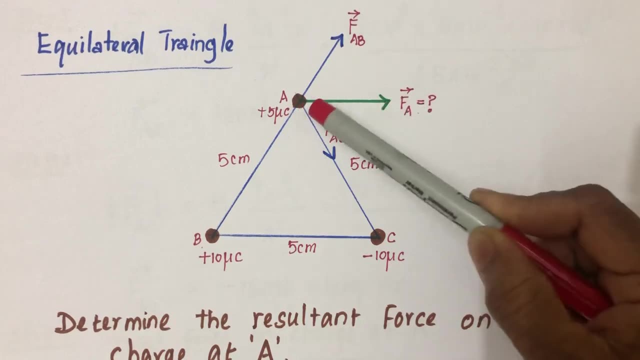 it will be a repulsive force, So it should go away like this. So let me show you how to do it. So let me show you how to do it. So let me show you how to do it. This is the force on A due to this negative charge: negative 10 microcoulomb. Okay, So it should be. 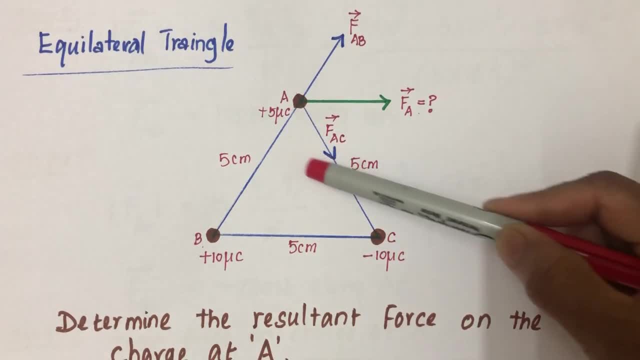 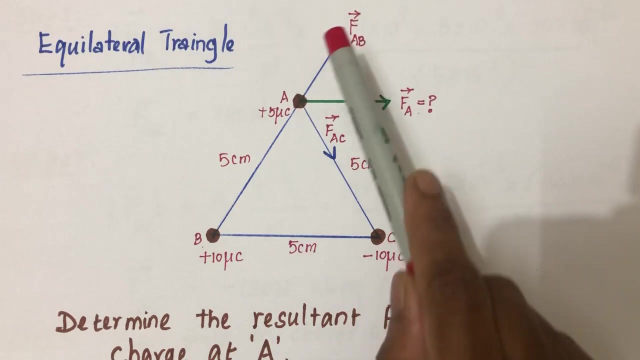 attractive force, So this charge will attract this in this direction. So this is the force acting on A due to this negative charge kept at C. Now we have to find out the resultant of these two vectors. So for that, first we have to find out the magnitude of FAB and then the magnitude of FAC. 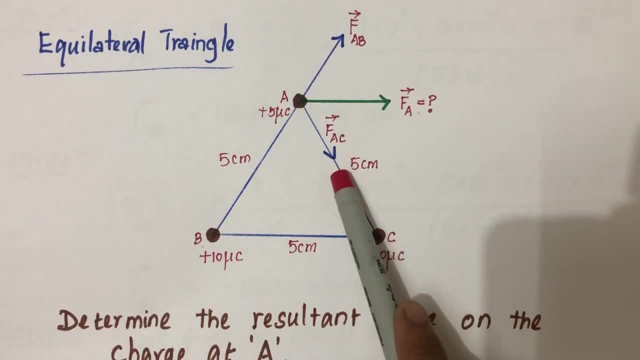 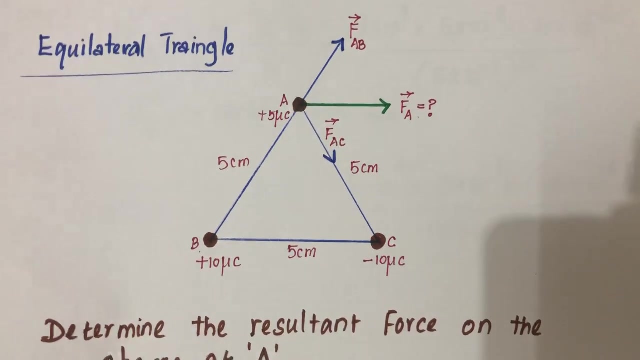 and then we are going to use the parallelogram law of addition and to find out the total force, that is, the resultant force acting at charge plus 5 microcoulomb, which is at A. okay, So the first step is to calculate. 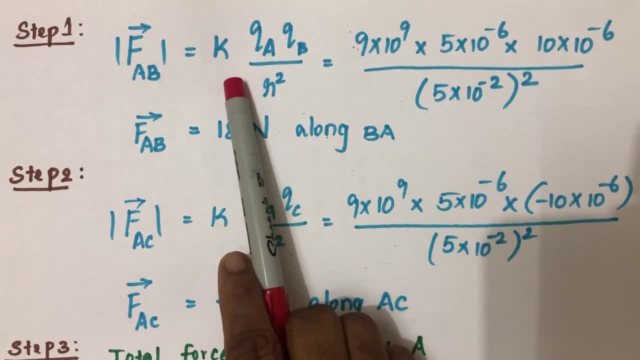 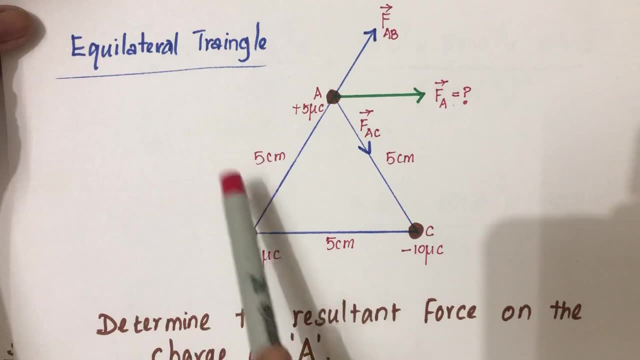 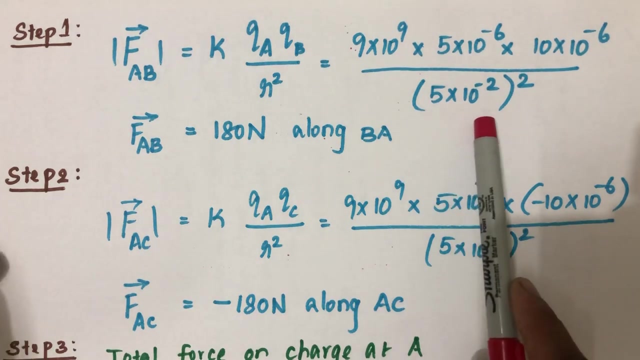 the magnitude of FAB. We know it is KQAQB divided by R square. okay, R is also given. since it is an equilateral triangle, all the sides are equal to 5 centimeter. So centimeter to be converted into meter. So 5 into 10 power minus 2, whole square. Please do not forget to square.